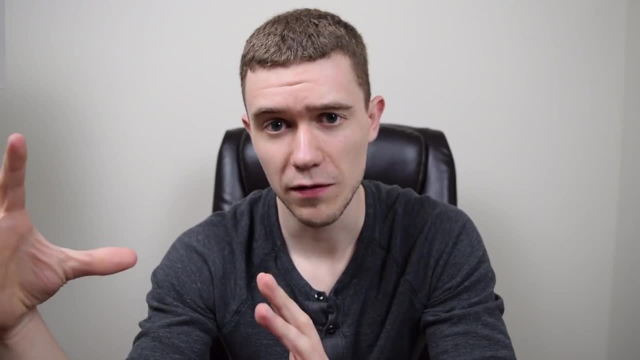 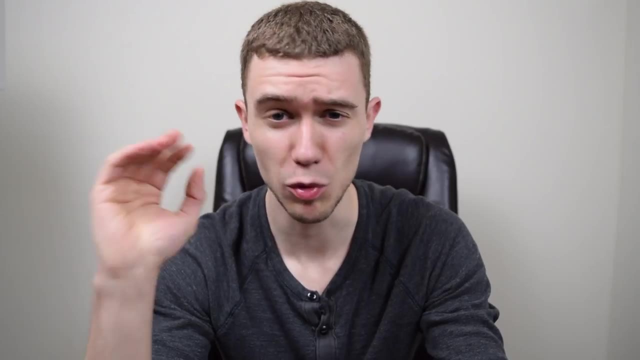 abilities and will test you on them. One thing I said in the previous video is that this isn't high school anymore. The level of rigor and expectation of ability is much, much higher than it will ever be in high school. You are in college now and you should expect things to be. 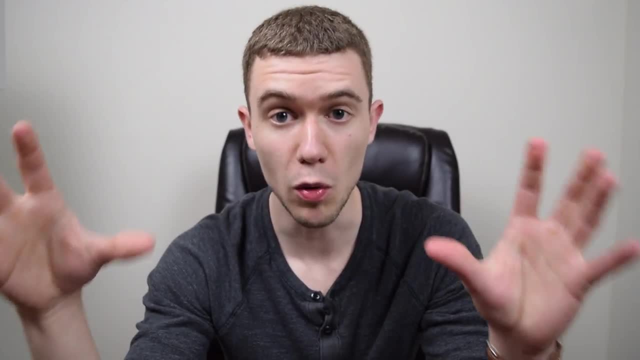 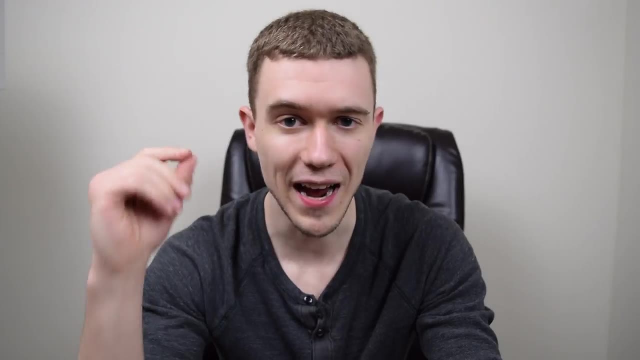 much more challenging and difficult. If you're finding that when you go in and take a test and it's nothing like you were expecting, that means you need to have a conversation with the professor. You need to ask them: hey, what exactly are you looking for? Which problem should I be doing to? 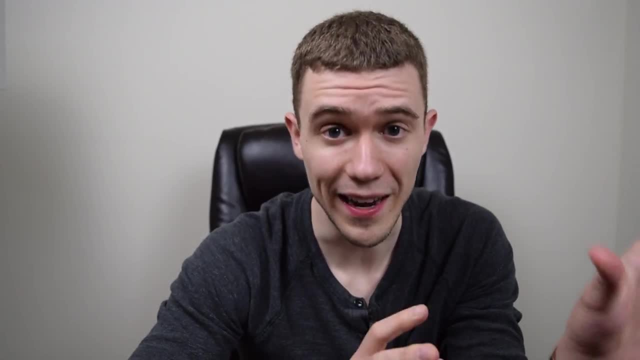 best prepare myself for the test? Are the tests going to be more like the lectures or like the homework? Do you have any samples of tests from previous years I could go over? The more you talk to the teacher, the more likely you are to get the test. The more likely you are to get the test. 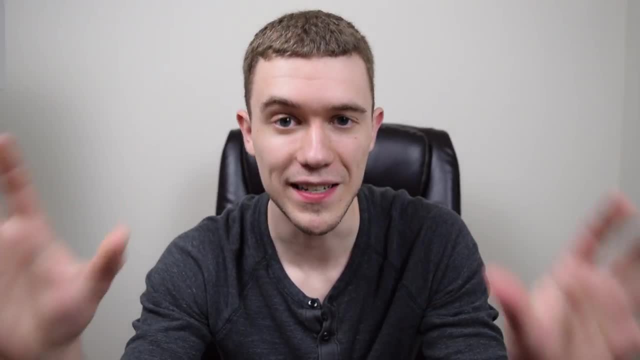 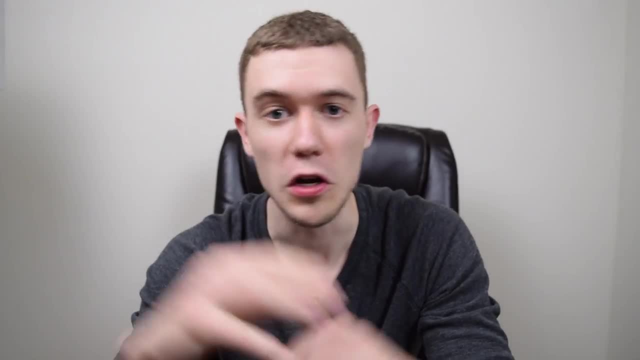 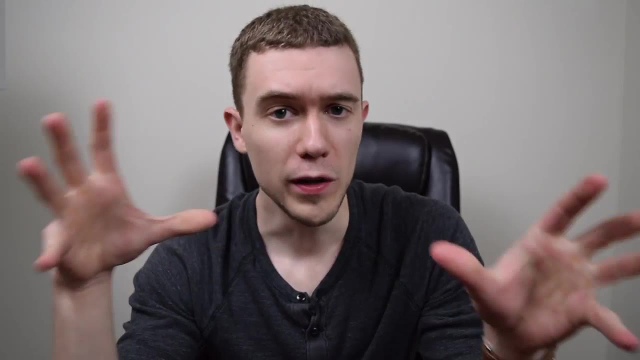 about what the tests are going to be like. Number two: you're not doing enough homework problems, or maybe you're not doing any homework problems, or maybe you're just not doing the right homework problems. Doing web aside or online homework is probably not enough A lot of times, what people do 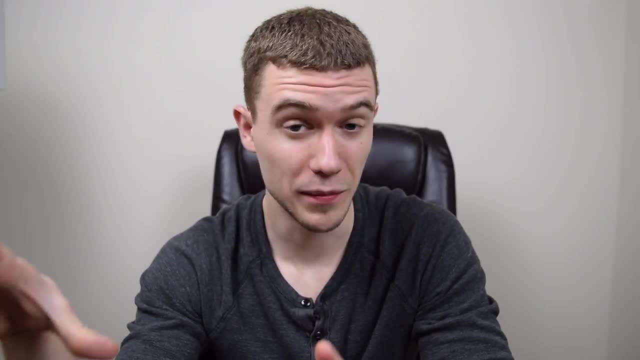 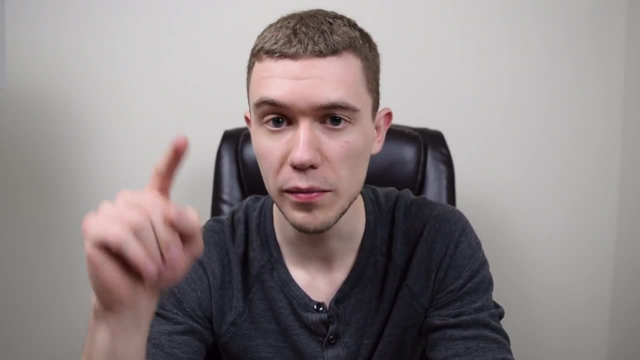 is they do web homework and maybe they're not even really doing them all themselves. It's really easy to get the answers offline, but nine times out of ten the web homework is nothing like the tests You should be doing- book problems. My recommendation is to do the assigned homework and more homework. 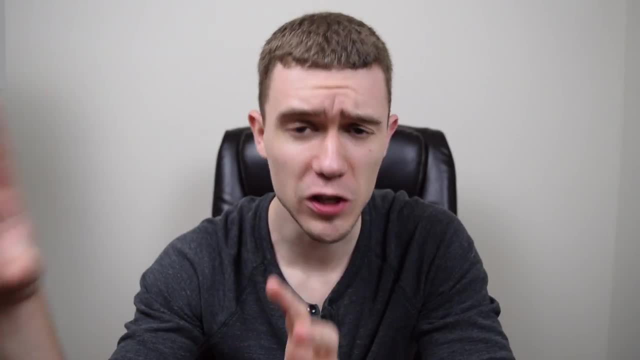 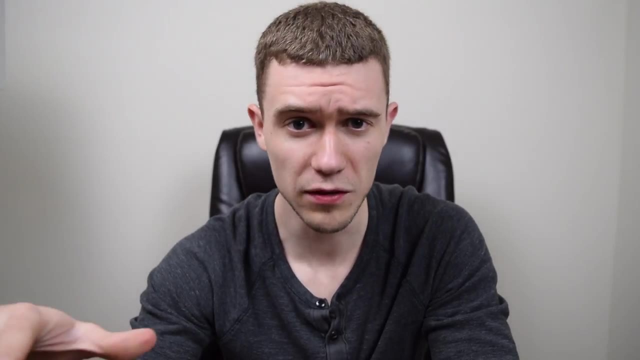 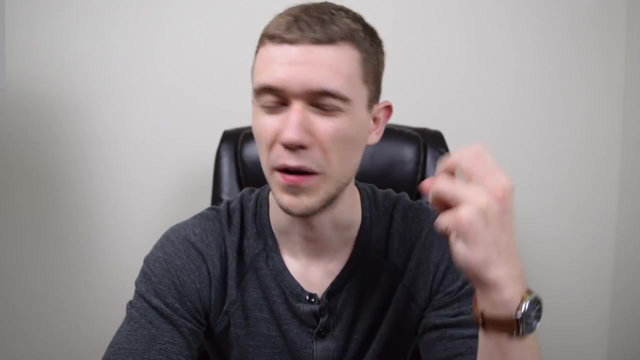 than was even assigned. Do problems from the ends of the chapter. Do the harder homework problems. If you can do the hardest book problems, the tests will be a total breeze for you. You learn math by doing math. You need to be doing problems or you will not be prepared for the tests. My third and 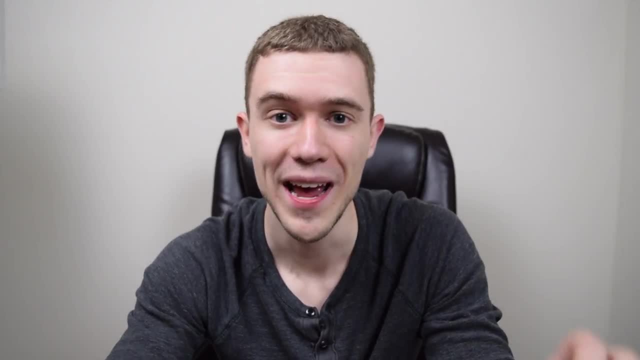 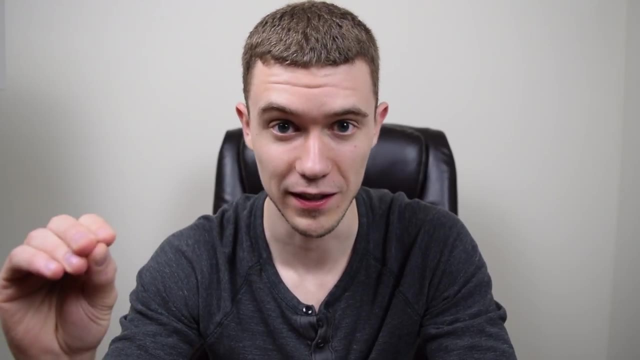 final tip. you probably know what it is if you've seen my last video. it's your algebra and trigonometry skills. So many people enter freshman calculus with poor algebra and trig skills. These are essential to your success in calculus. I can't stress this enough. If you're making algebra or 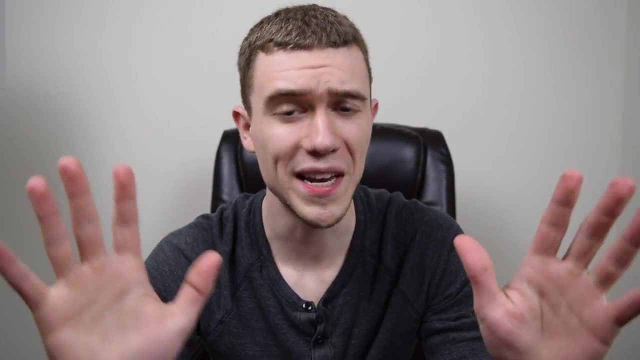 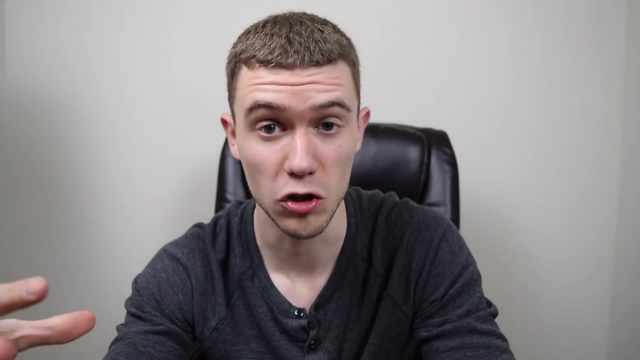 trig mistakes. review that material. It won't take you as long as you think. You have to know properties of exponents and logarithms and fractions and evaluating trig functions, trig identities and trig functions. If you're not familiar with trig functions, you should know.